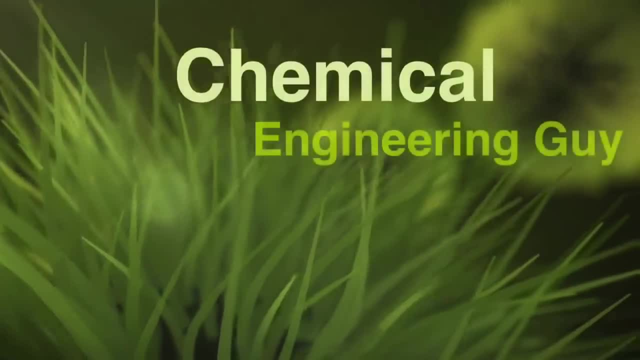 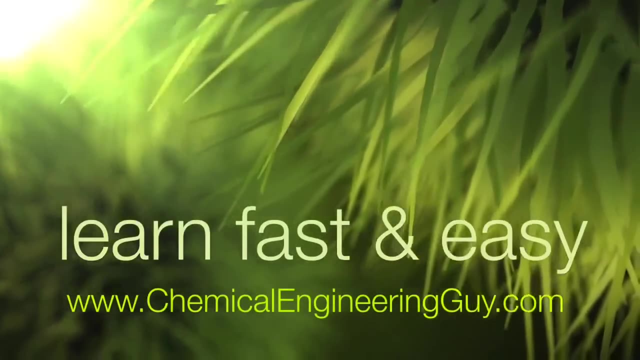 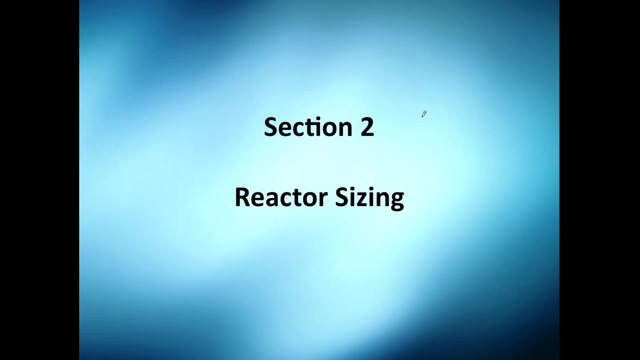 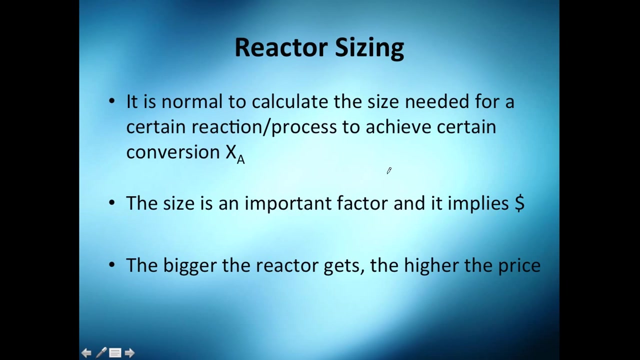 So we're done with section number one. let's continue section number two, which is reactor sizing. Now, what's reactor sizing? It's essentially calculate the size needed for a certain reaction or process to achieve certain conversion. So generally, you choose or set conversion. 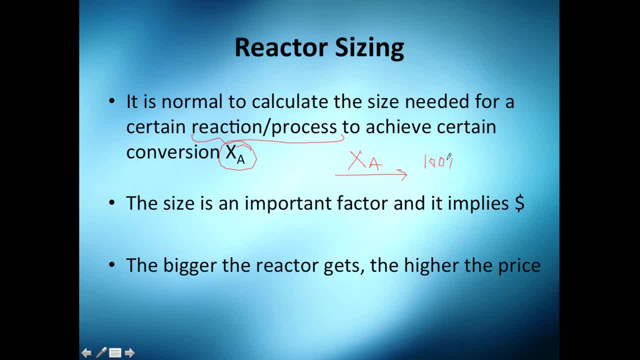 probably you want the highest. let's say 100% if it's possible, or maybe the most convenient one is 20%, given, I don't know, operation cost, temperature impossible to achieve, or a catalyst is way cheaper. whatever You choose, the conversion you want, and once you choose, 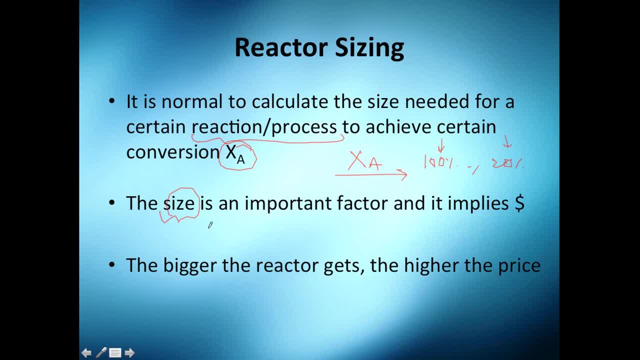 the conversion. you size your reactor. So one thing here is: the bigger the size or the bigger the reactor gets, the higher the price. So that's one other thing. For example, you want 90% conversion. maybe you got, I don't know, 100 cubic meters And you want to change this to 99, maybe I don't. 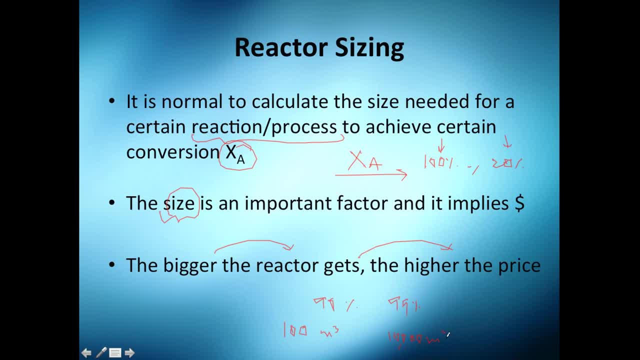 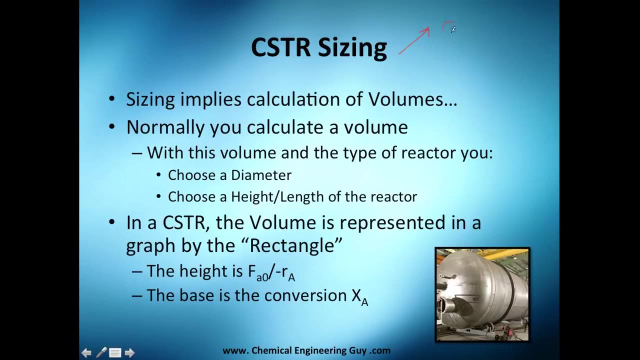 know it's not linear. you will need 10,000 cubic meters just to improve 9%. Well, I think it's not worth it, So you're probably going to stick with this. Okay, now let's continue with the continuous-stirred tank reactor. We're going to see only two. 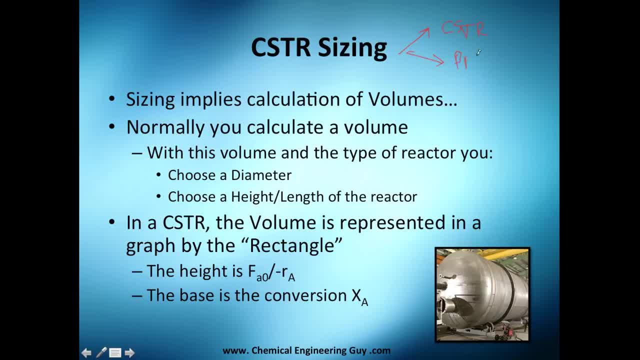 CSTR, which are the two most classic, and the PFR, the continuous-stirred tank reactor, which, thank God, it's arithmetic, not a differential or integral form, And we got the PFR. actually, this is more like a tube. 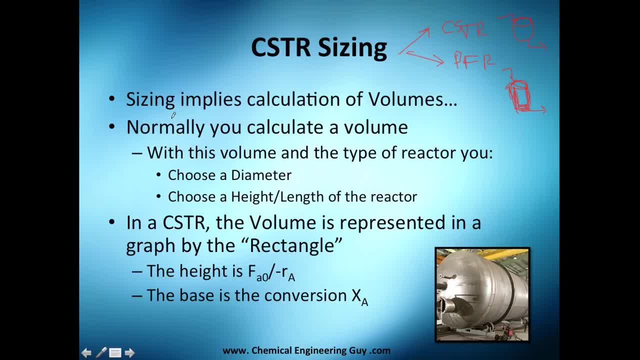 But you get me. Let's see CSTR. The sizing implies calculation of volumes. Of course sizing means size. Normally you calculate the volume given the conversion and the flow conditions and the rate of reaction or type of reaction And with this volume you go to typical ways to. 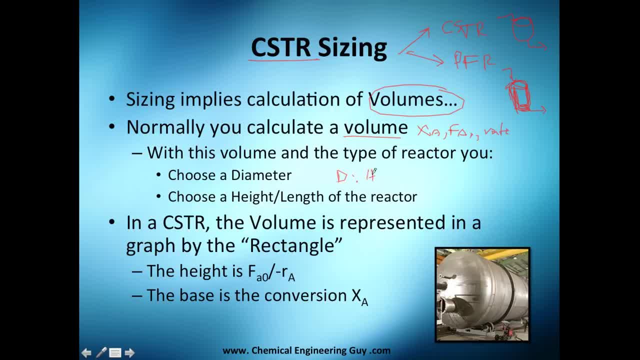 choose its diameter to height or those type of ratios. So you choose a diameter and you choose a height if you're doing a tank, or a length if you're doing a pipe. We're not going to do that in this course, but just to let you know it's normal that. 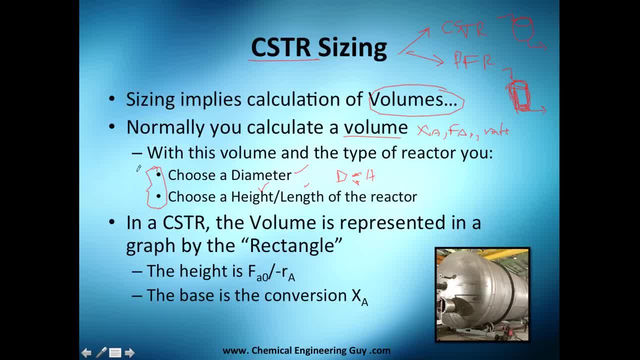 a chemical engineer do that. So I think this is in chemical plant design. you're going to see those heuristics or those values or rules or thumb rules to get the size of the reactor. Now, In a continuous-steer tank reactor, the volume is represented in a graph, or let's say in: 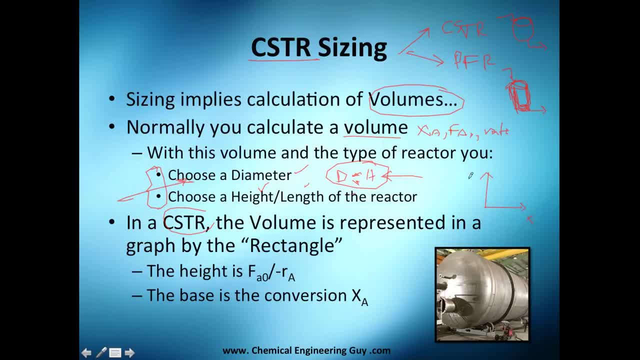 a conversion here and a rate of reaction here. Of course, multiply by flow, It's by a rectangle. so you get this, you get this. and the area here, this area in the graph, is my volume, So it sounds kind of crazy. 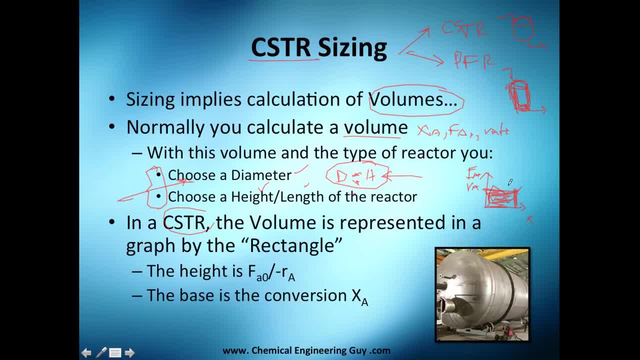 Say that the volume is actually the area, you will say no, the area. you need to still multiply it by a height to convert it into volume. but we're talking about this concept here. We're going to see it later. so just trust in me and trust that that rectangle is that. 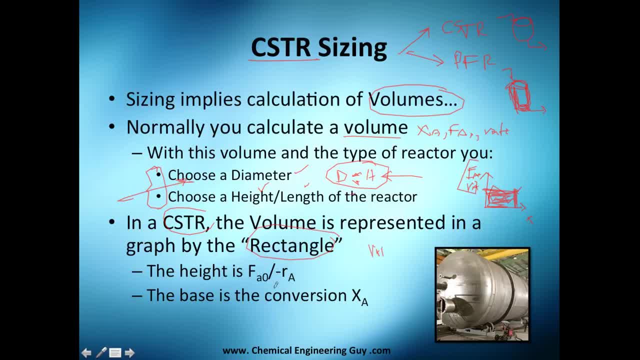 area is the volume or the total volume needed. So the height I'm talking about in this rectangle is this height, which is the amount of, or the flow of A at the beginning divided by the rate of reaction in that area. So that's what I'm talking about. 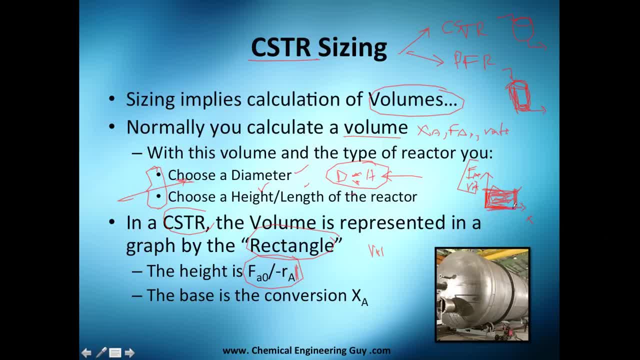 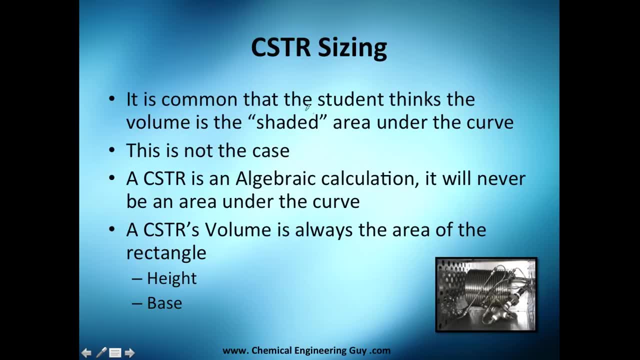 The volume is the conversion and the base is the conversion. Now it is common that the student thinks the volume is the shaded area of under the curve. So once again I got this and many people or students because they have seen I don't. 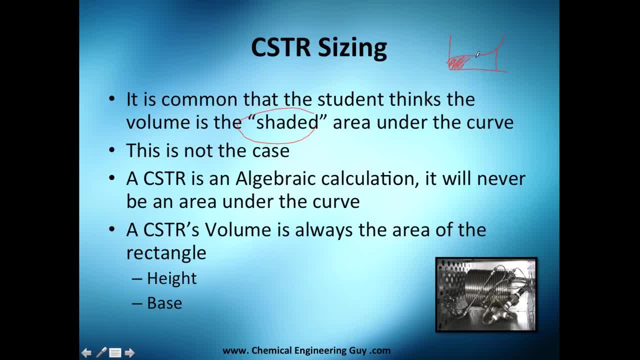 know mathematics, or so they tell me that the volume should be this area right here, And I tell you: no, that's not the case. You need to do this. It's more about the rectangle rather than the shaded area under the curve or the function. 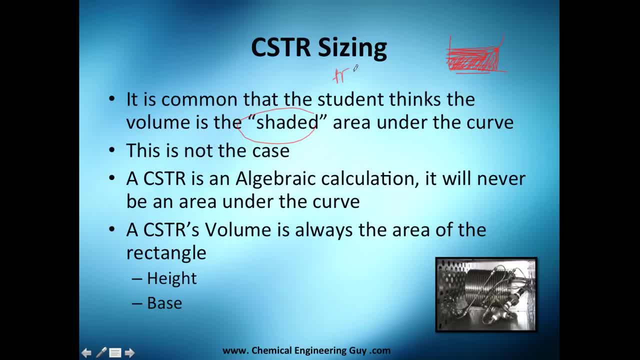 We're going to see that there is a special case for PFR, which, the student is right- is actually the area under the curve. But right now, just let's stick to the algebraic calculation. It's just a rectangle. You have one height and you have one base, which is actually conversion and the rate. 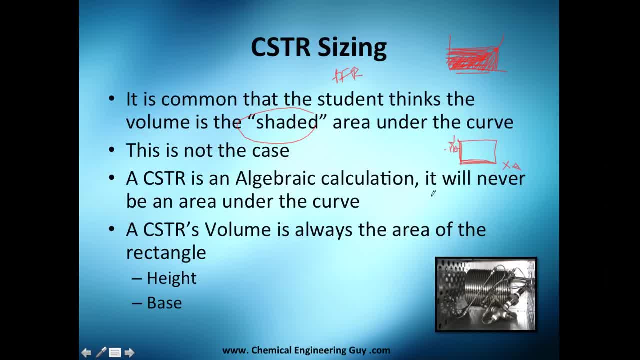 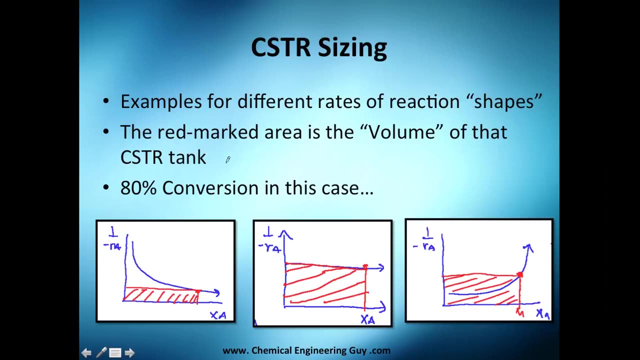 of reaction here. And yeah, Yeah, Once again, it's a rectangle with a height and a base, So I'm going to show you some examples for these, let's say, different shapes of rate of reaction, The red marked area or these lines. in theory it's an area, but okay, yeah, maybe it's strange. 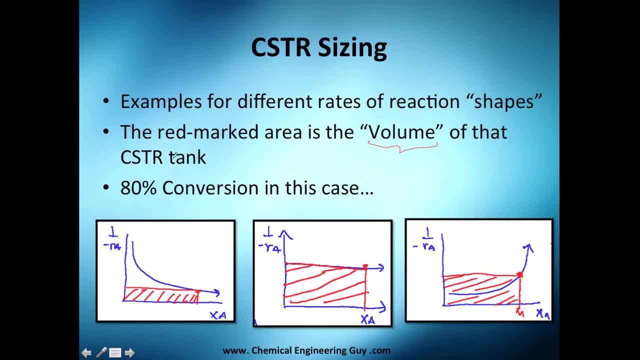 for you is the volume of that CSTR tank or reactor. So I use 80% conversion in all cases. This line right here is the rate of reaction. How would you plot the rate of reaction? You cannot see this one here, but it's just a straight line here. 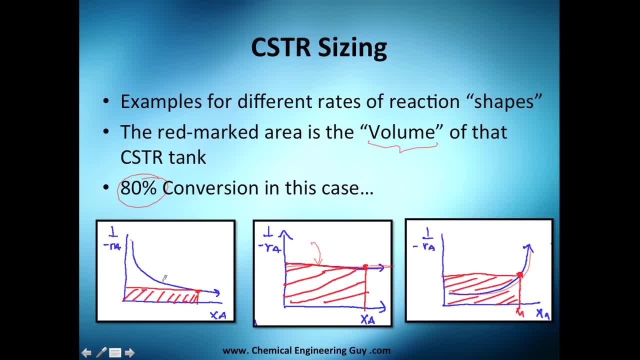 And this one is increasing. So just imagine this is the rate of reaction, or the inverse, or one divided by the rate of reaction, And what I'm telling you about, guys, is that the volume of that reactor will depend on the shape. And where do you get it? 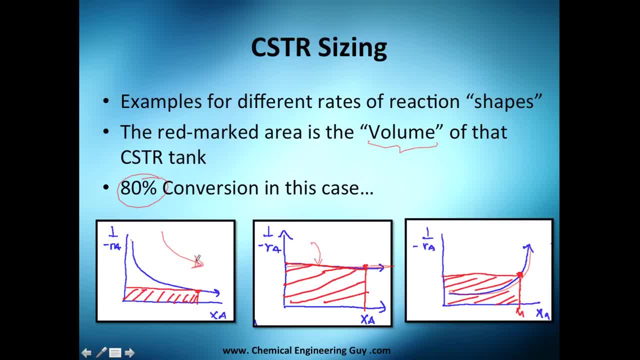 So, for example, I got this shape Or this rate of reaction. I choose the 80% because this is my 80%. So I stick it here and see where I intersect with my rate of reaction And then make a horizontal line. 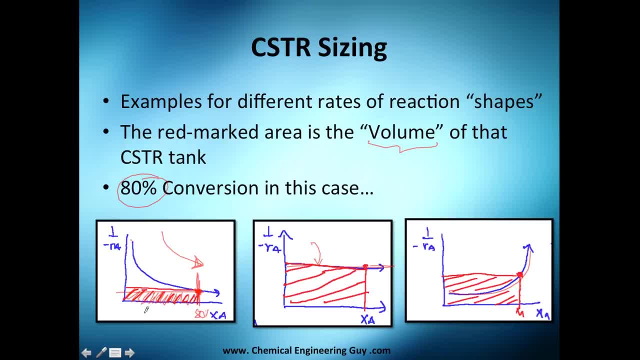 And I will get this. This shaded area- I don't know. let's say it's 1.5 cubic meters- will be the volume of that CSTR with that rate of reaction and that conversion. The same thing goes here: 80% is here. 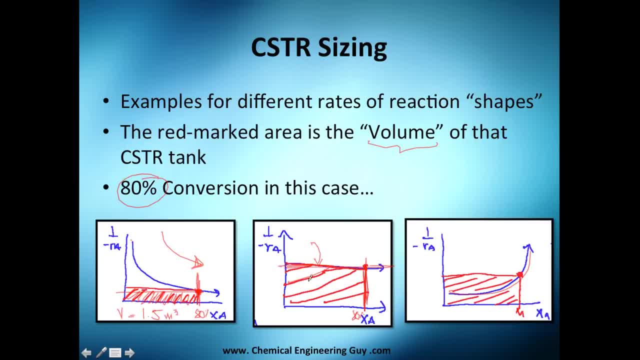 Then stick it here and do a horizontal line. Since the rate of reaction plot is already a horizontal line, well, it doesn't make any difference. This is actually the only case in which the area under the function or under the curve is what the student told: the volume. 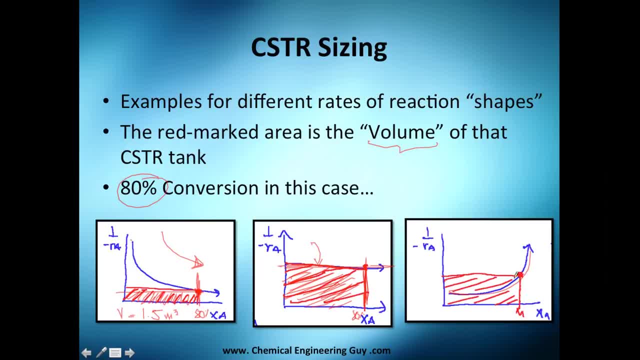 And last but not least, as you can see, this one goes up And you choose the 80% here, So you drop it here, And then you Once again do a horizontal line, And all this will be your volume. 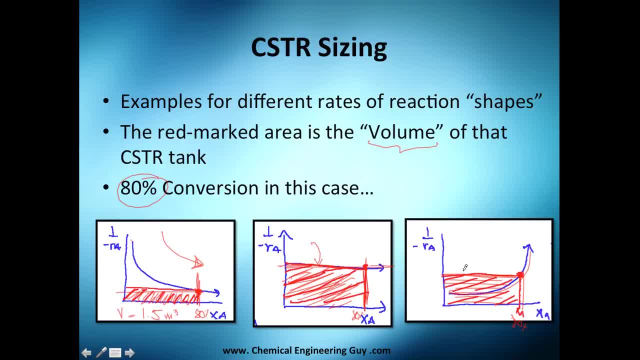 Why I'm telling you this, guys? because probably you have no idea right now. but you're going to see that when you start calculating the bigger or the sometimes you calculate a volume of CSTR and you get lower volumes. You calculate it and you get high volumes. and you will be asking or wondering yourself: 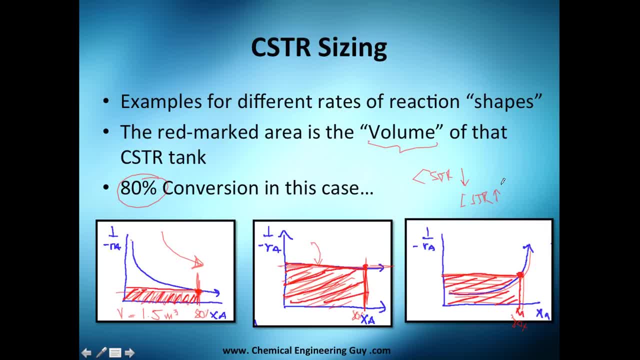 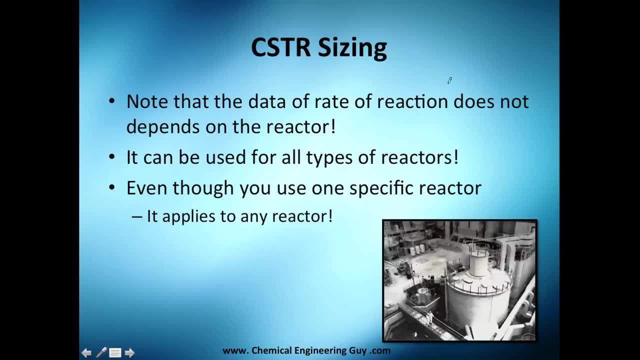 on what does that depend? So this is the answer to that. Well, once again, the data of rate of reaction- that is the shape of my plot. we've seen it before are going up- does not depend on the reactor. 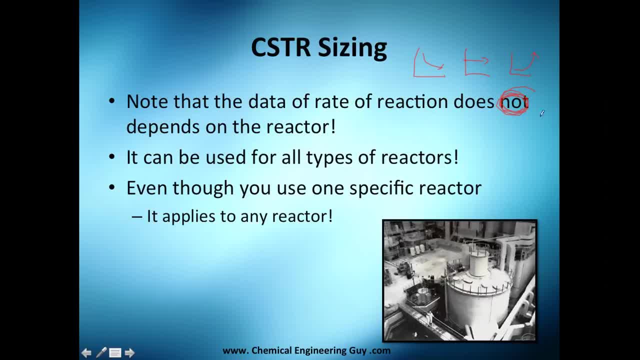 So, once again, the rate of reaction does not depend on the reactor. So I could choose a PFR, I could choose a PBR, I could choose a- I don't know- a CSTR, any tank or any reactor I can imagine. 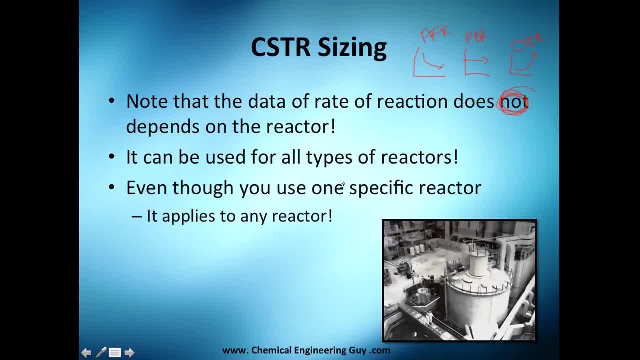 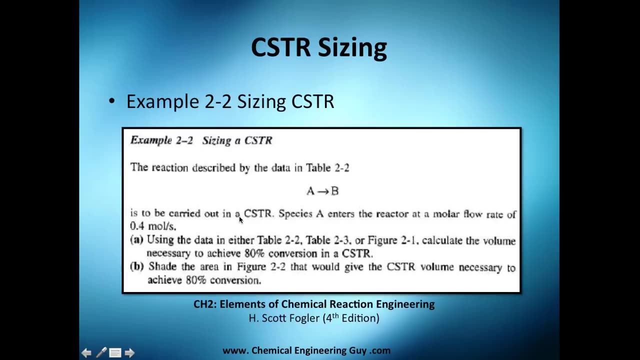 And the rate of reaction is dependent on the reaction, not on the reactor. The good thing is that we can actually get one and apply it for any other reactor. So, once again, it applies for any reactor, And I think we're going to do this example in the other video. 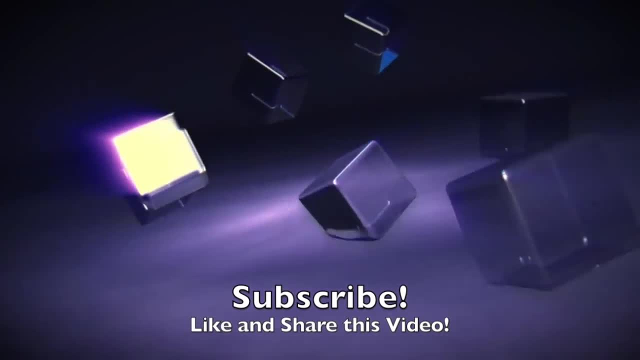 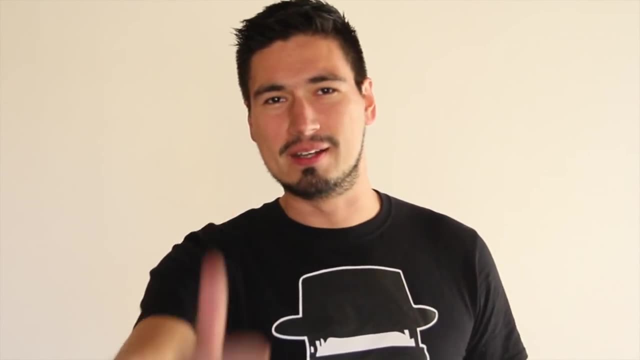 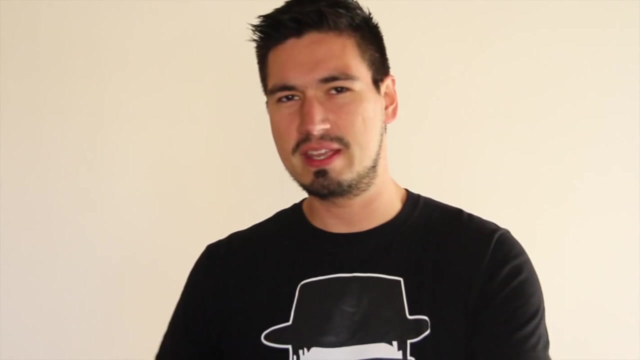 What's up guys? it's me, Chemical Engineering Guy. so if you liked the video, why not push the like button? It really helps me to know if you're liking the videos or if I should be changing something or I should be adding something, taking out content, whatever. 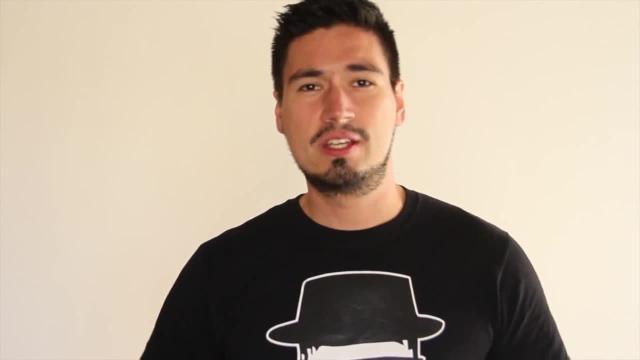 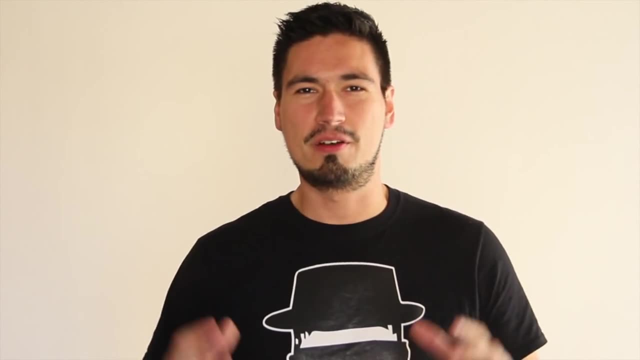 Also, sharing is caring. So if you've got any kind of friends, teachers, colleagues or whatever kind of person that might be interested in this type of content, why not share it? Sharing helps you out. It helps our community to grow faster- in members and in content. 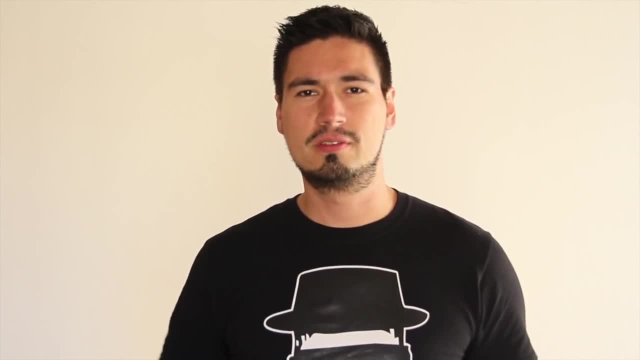 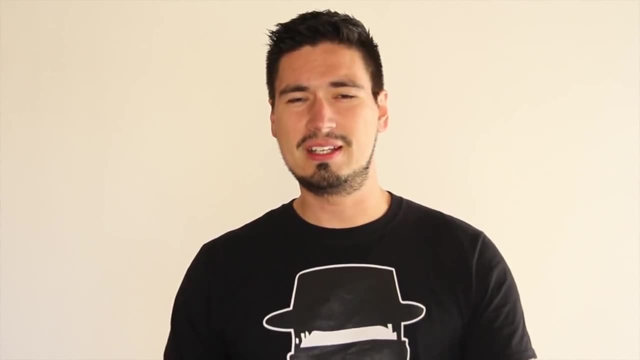 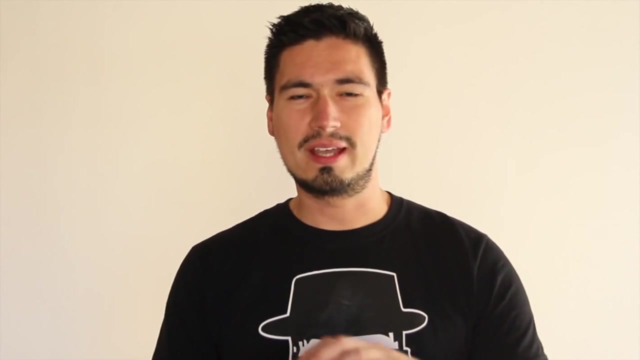 If you want to keep track of my activity- videos, uploads, experiments, playlists, whatever content I'm getting on YouTube- be sure to click the subscribe button. Subscribing to the channel is totally free, guys. My dream is to create an online academy of chemical engineering where everyone can access.